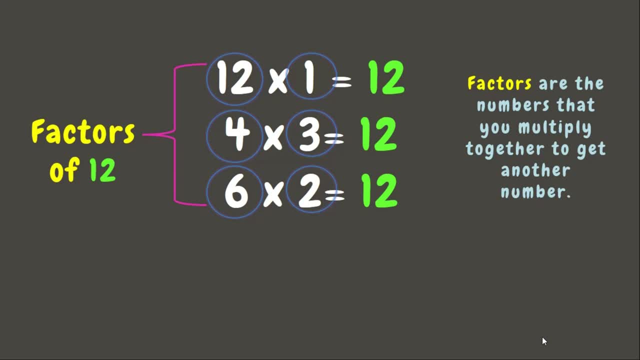 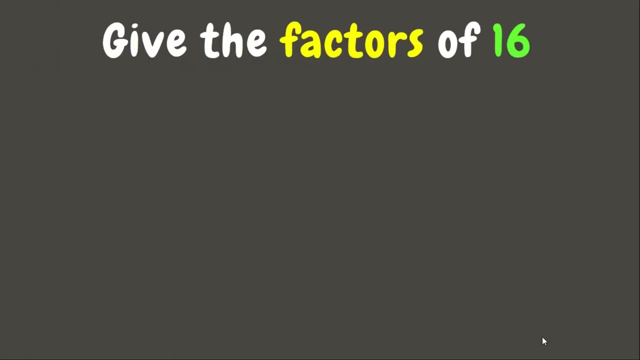 that you multiply together to get another number. Therefore, the factors of 12 are 12,, 1,, 4,, 3,, 6, and 2.. Let's have another example: Get the factors of 16.. Let's list it down: 16 times 1. 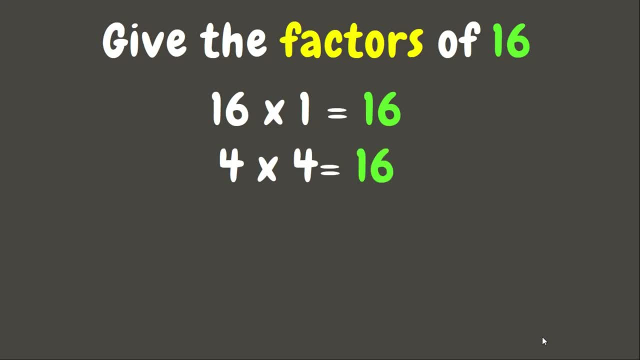 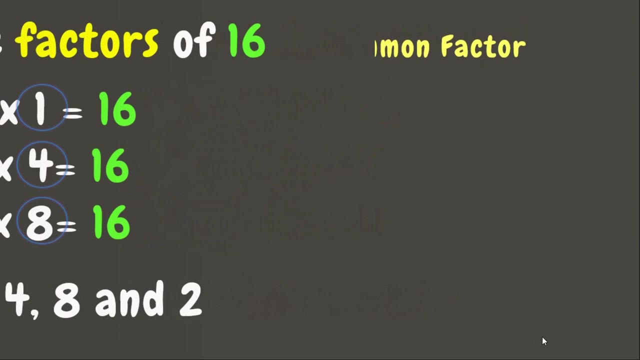 equals 16.. 4 times 4 equals 16.. 2 times 8 equals 16.. So the factors of 16 are 16,, 1,, 4,, 8, and 2.. Great job, Now that you know what are factors. 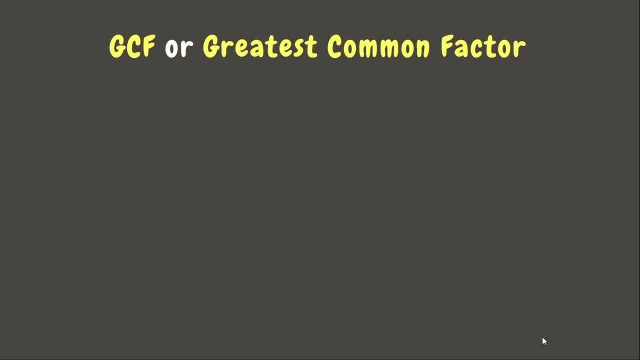 let us now proceed to GCF, or greatest common factor. Can you give the greatest common factor of 6 and 9?? First let's list down the factors of each number. The factors of 6 are 6,, 3,, 1,. 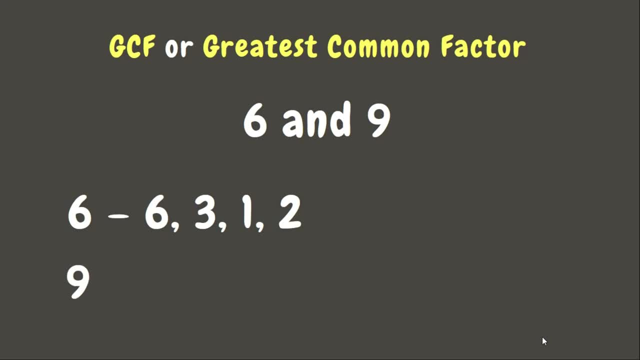 and 2.. While the factors of 9 are 3,, 1, and 9.. Look at these factors. Can you see? what are their common factors? Very good, Their common factors are 3 and 1.. When we say common, that is same or 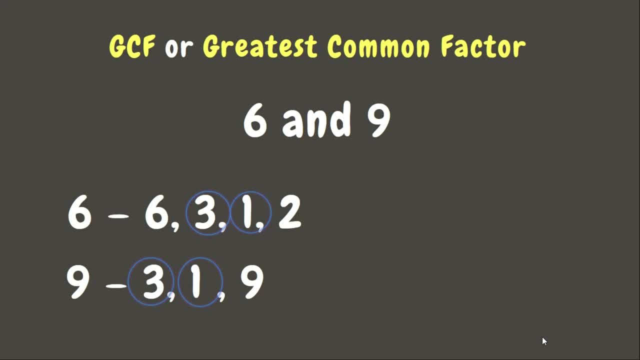 similar, But we are only looking for the greatest common factor. Greatest means pinaka malaki. Ano, ang pinaka malaking parehas ng factor nila? Good job, It is number 3.. Therefore, the GCF of 6 and 9 is 3.. Let's have one more. Let's find the GCF of 8 and 2.. The factors of 8 are 4,, 2,, 1, and 8.. 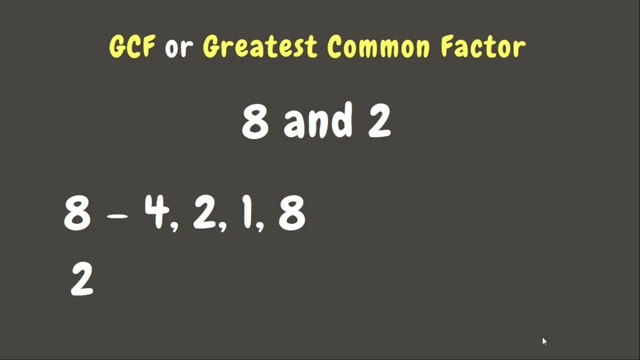 while the factors of 2 are 2 and 1.. The greatest common factor is Very good, It is 2. Wonderful. Now let's try to get the GCF of this concept. How to get the 8 and 1?? 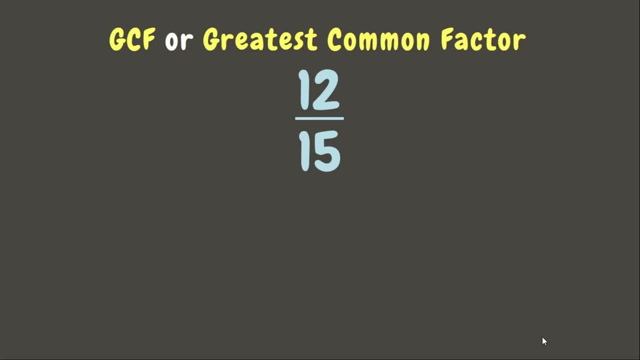 Collect formula for y numbers: 1 minus y minus 5 times 6.. How to get the fraction? Let's get the factors of the numerator and the denominator. The factors of 12 are 12,, 1,, 3,, 4,, 6, and 2. While the factors of 15 are 15,, 1,, 3,, 5.. 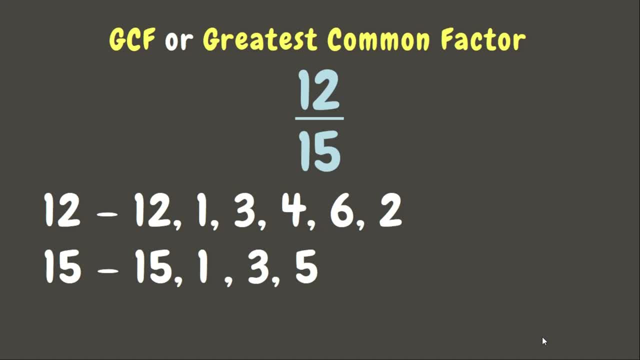 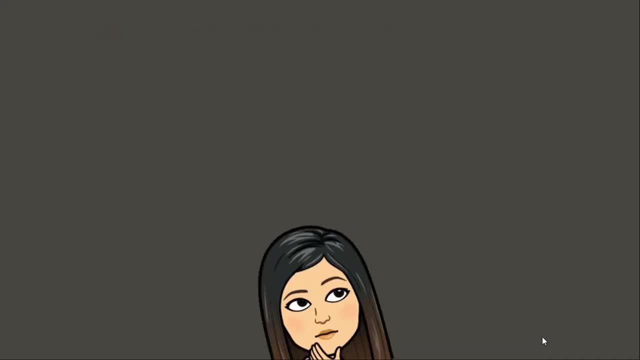 Their common factors are 1 and 3, but their greatest common factor is 3.. Now we are already done with the GCM. Now it's time for us to learn how to get the least common multiple, or LCM. But what is multiple? Let's look at this one. What? 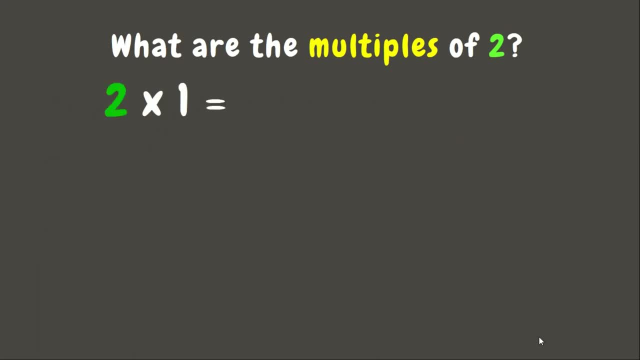 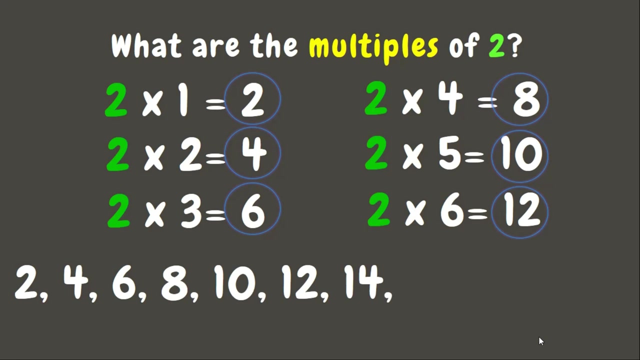 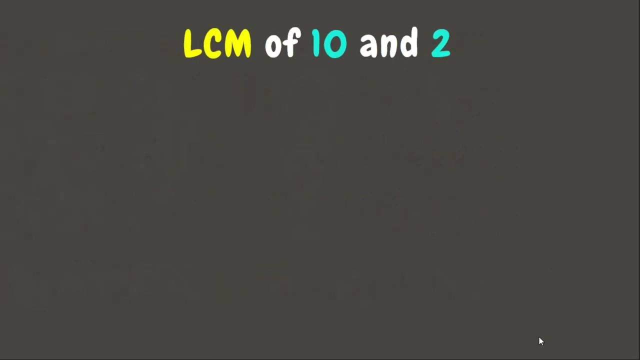 are the multiples of 2?. These numbers are what we call multiples. The multiples of 2 are 2,, 4,, 6,, 8,, 10,, 12,, 14,, 16,, 18,, 20, and so on. Now let's try. 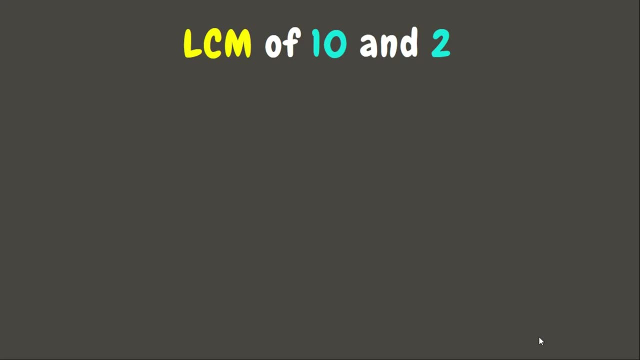 to get the LCM, or least common multiple of 10 and 2.. First let's list down all the multiples of each number. The multiples of 2 are 2,, 4,, 6,, 8,, 10,, 12,, 16,, 18,, 20, and so on. 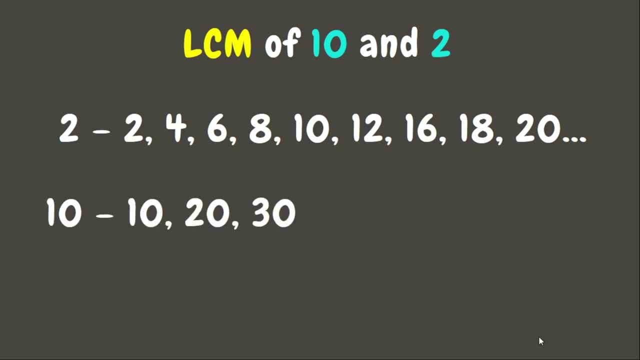 The multiples of 10 are 10,, 20,, 30,, 40,, 50,, 60, and so on. Remember, hindi nati kailangan isulat lahat ng multiples. Now let us circle all the common. 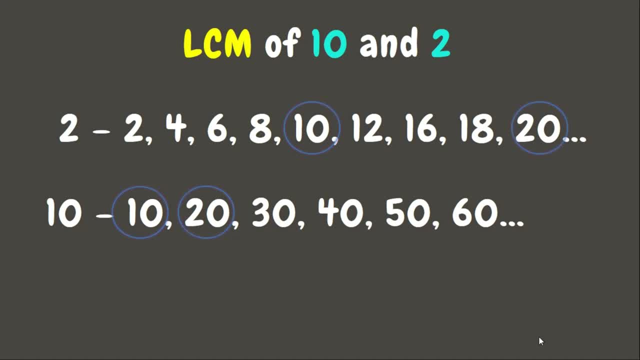 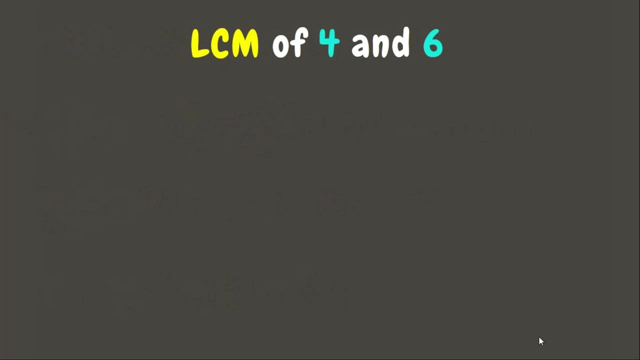 multiples 10 and 20.. But we are only looking for the least Pinakamaliit na parehas sila, And that is 10.. Therefore, the LCM of 10 and 2 is 10.. Let's have another example.